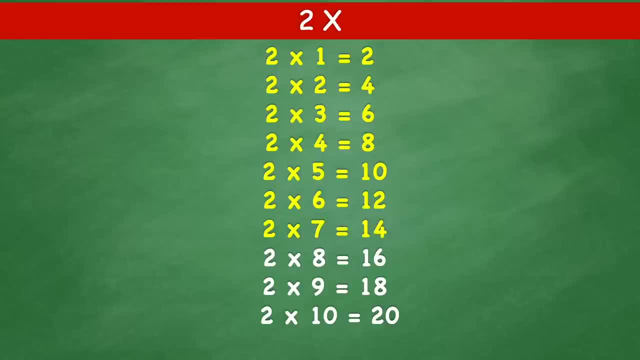 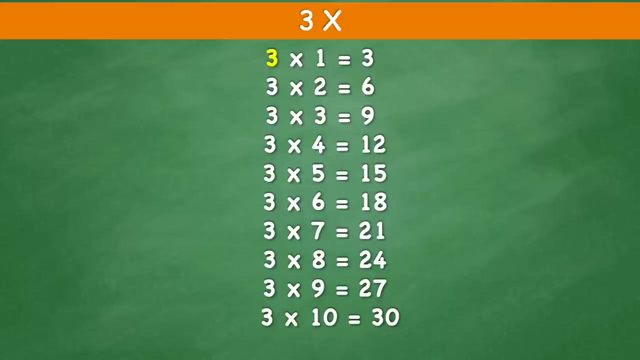 2 x 7 equal 14. 2 x 8 equal 16. 2 x 9 equal 18. 2 x 10 equal 20. 3 x 3 x 1 equal 3. 3 x 7 equal 8. 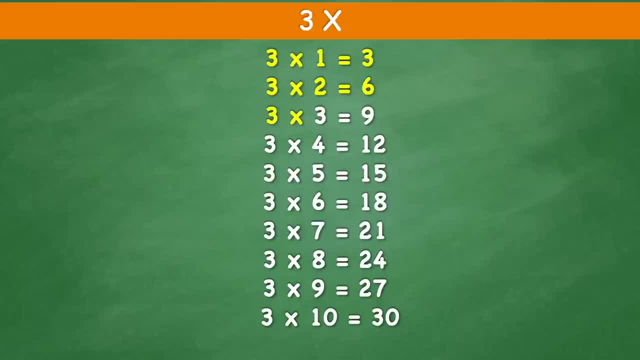 3 x 7 equal 9. 3 x 8 equal 12. 3 x 9 equal 12. 3 x 9 equal 15. 3 x 10 equal 17. 3 x 10 equal 18. 3 x 11 equal 17. 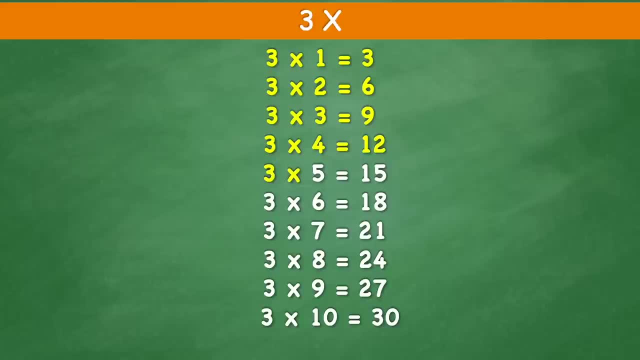 3 x 12 equal 18. 3 x 12 equal 18. 3 x 13 equal 19. 3 x 13 equal 19. 3 x 14 equal 19. 3 x 14 equal 20. 3 x 15 equal 19. 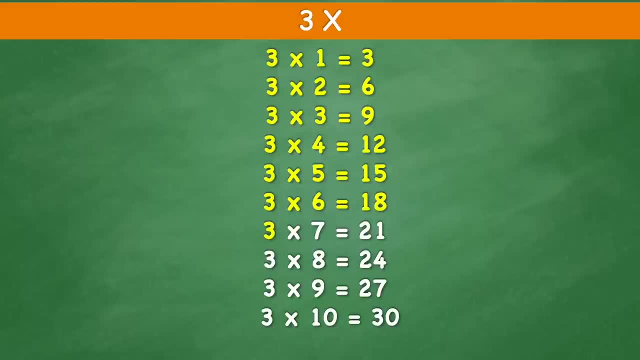 3 x 16 equal 20. 3 x 16 equal 19. 3 x 17 equal 20. 3 x 18 equal 19. 3 x 17 equal 21. 3 x 18 equal 21. 3 x 18 equal 24. 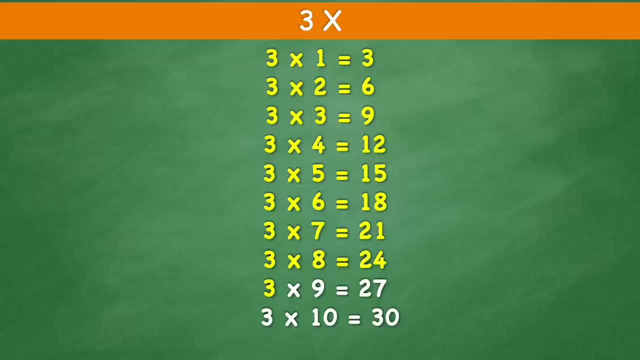 3 x 19 equal 24. 3 x 20 equal 24. 3 x 21 equal 24. 3 x 22 equal 24. 3 x 23 equal 24. 3 x 23 equal 24. 3 x 23 equal 24. 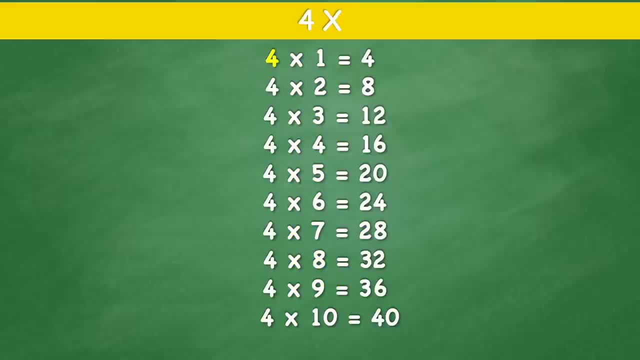 3 x 24 equal 24. 3 x 25 equal 24. 3 x 28 equal 28. 3 x 30 equal 30. 4 x 1 x 4 equal 4. 4 x 1 equal 0. 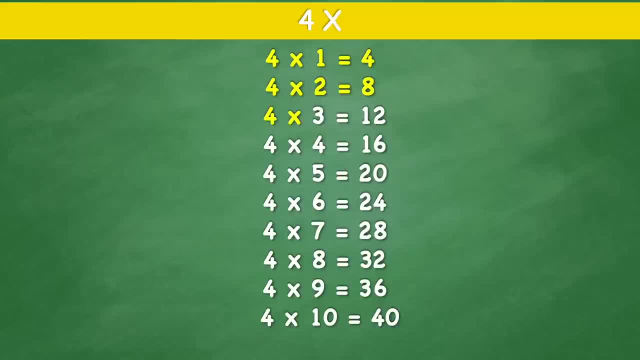 4 x 2 equals 0. 4 x 13 equals 12. 4 x 4 equal 16. 4 x 5 equals 20. 4 x 6 equals 24. 4 x 7 equals 28. 4 x 8 equals 17. 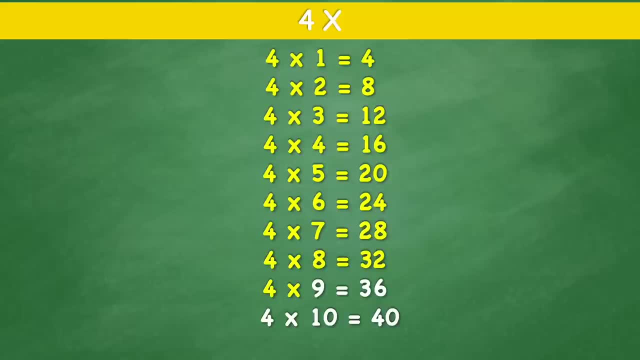 times 8 equals 32. 4 times 9 equals 36. 4 times 10 equals 40. 5 times 5 times 1 equals 5. 5 times 2 equals 10. 5 times 3 equals 15. 5 times 4 equals 20, 5 times 5. 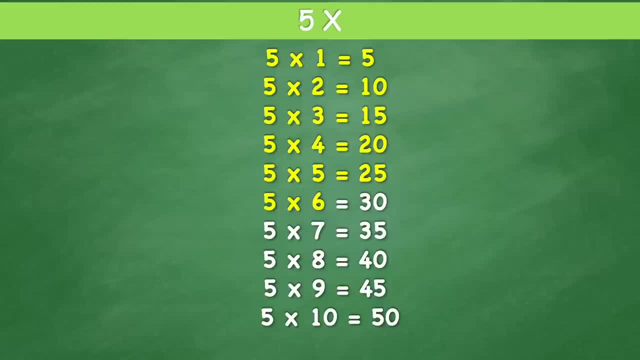 equals 25, 5 times 6. equals 30, 5 times 7. equals 35, 5 times 8. equals 40, 5 times 9. equals 45, 5 times 10. equals 50, 6 times 6 times 1. equals 6, 6 times 2. equals 12. 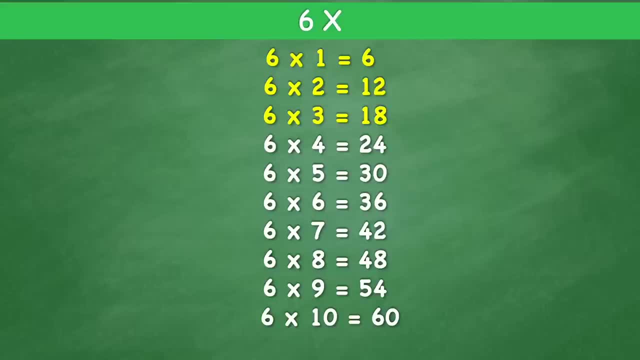 12 six times three equal eighteen. six times four, equal twenty four six times five equals thirty six times six equal thirty six. six times seven equal forty two, six times eight, equal forty. eight. six times nine equal fifty four. six times ten equals sixty seven times seven times one equals. 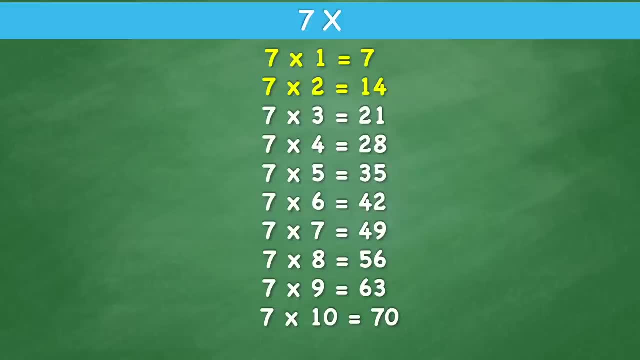 seven seven times two equal fourteen. seven times three equal twenty. one. seven times four equal twenty. eight. seven times five equals thirty five. seven times six equal forty two. seven times seven equals forty nine. seven times eight equals fifty. six. seven times seven equals sixty three. seven times ten equals seventy. 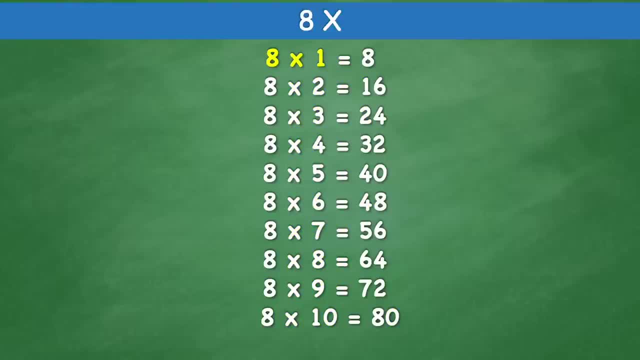 eight times eight times one equal eight. eight times two equals sixteen. eight times three equals 24.. eight times equal 32.. 8 times 5 equal 40.. 8 times 6 equal 48.. 8 times 7 equal 56.. 8 times 8 equal 64.. 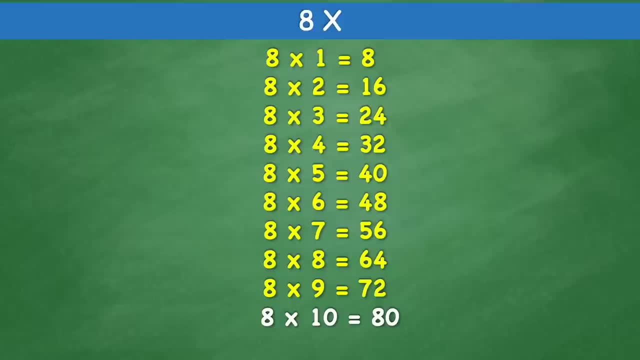 8 times 9 equal 72.. 8 times 10 equal 80.. 9 times 9 times 1 equal 9.. 9 times 2 equal 18.. 9 times 3 equal 27.. 9 times 4 equal 36.. 9 times 5 equal 45..